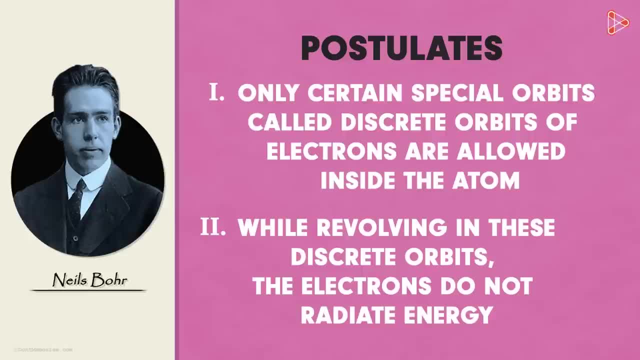 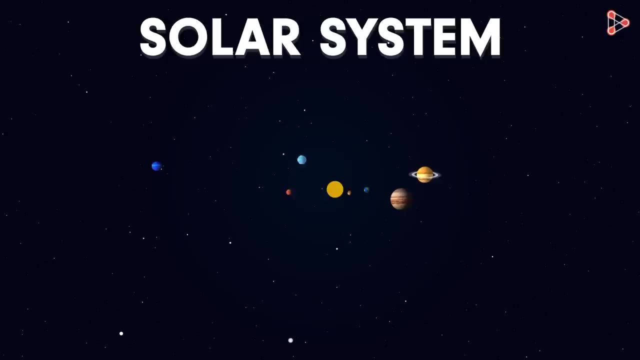 Now, these points definitely tell us why an atom is so stable. But what exactly are these paths or orbits in which the electrons revolve around the nucleus? Let's understand with an example. Do you know how our solar system is? Yes, it appears somewhat like this. 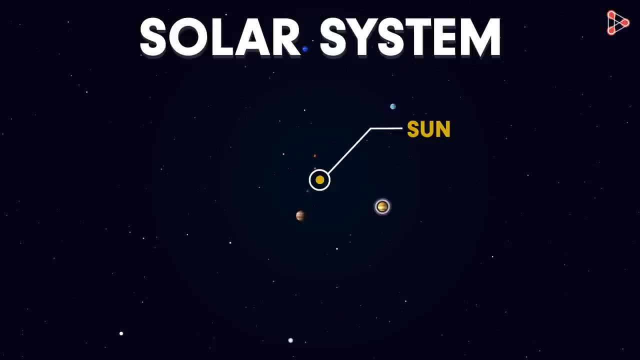 Now here, the Sun is stationary at the centre while the planets revolve around it. But have you noticed that the planets always revolve in fixed paths? We never find any planet jumping to a different path all of a sudden right. They always encircle the Sun in defined paths. 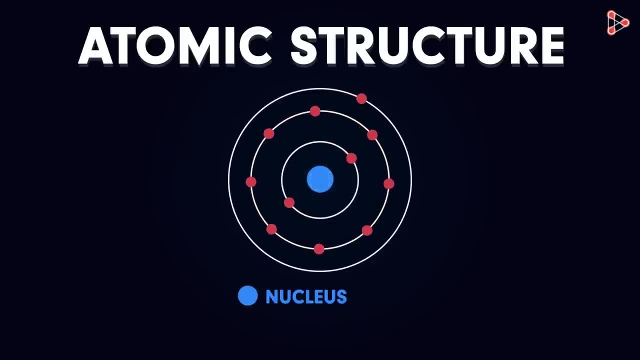 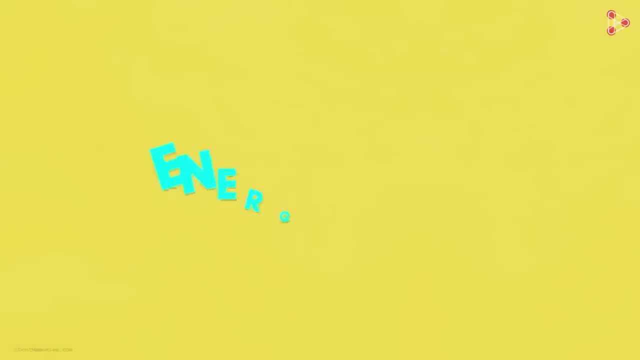 In a similar way, we have the atomic structure. The nucleus acts like the Sun, located at the centre, And the electrons are like planets, which revolve in fixed, defined orbitals. These electron orbitals are referred to as shells or energy levels. Now, the name energy levels gets us to an important concept. 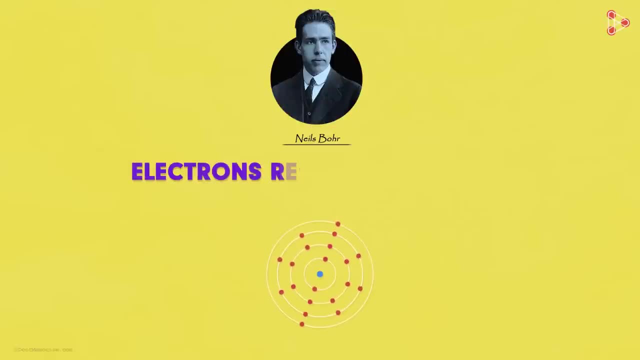 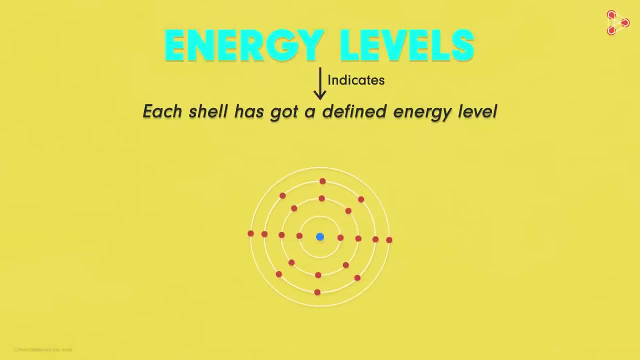 Niels Bohr suggested that the electrons revolving in these orbitals do not radiate energy. This is justified when we use the term energy levels, Because it indicates that each shell has got a defined energy level. That means when the electrons revolve in these shells, they do not liberate any form of energy. 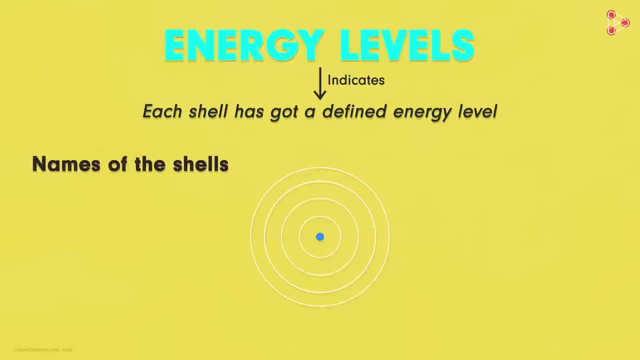 And how do we name these shells to indicate their position? It's simple: Beginning from the one near the nucleus, we name them as the K shell, L shell, M shell, N shell, and so on. Yes, K, L, M, N, and so on. 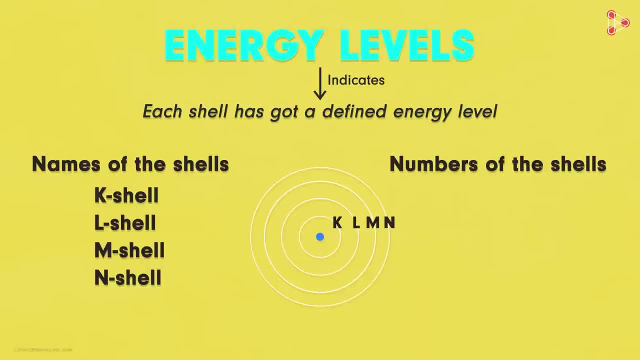 And what if we want to number them? In that case we use the letter N in lowercase and write them as: N equals 1, N equals 2, N equals 3, and so on. END, so on, beginning from the one next to the Nucleus. 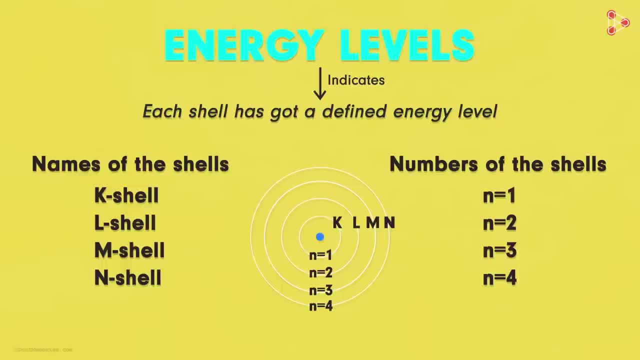 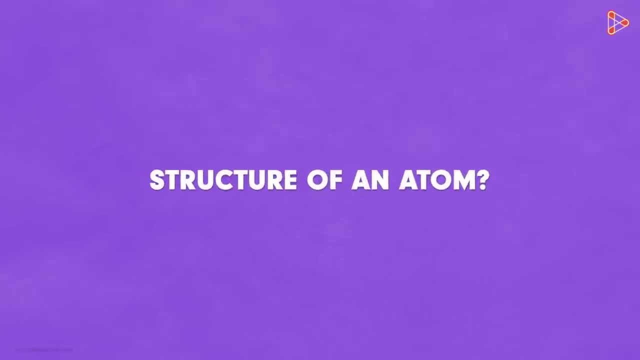 So we can name them alphabetically or we can even number them. With all these theories and points known, do we now know the structure of a typical atom completely? The Nucleus contains positive protons and the electrons revolving around in fixed orbitals. 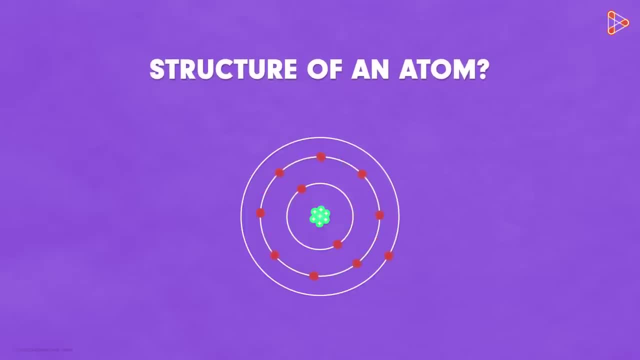 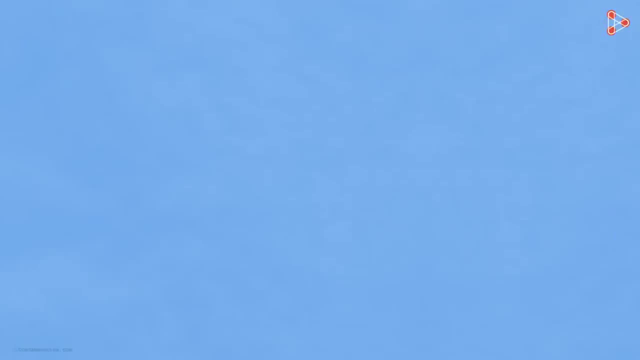 Is that how an atom is structured? Not really. We still have one more sub-atomic particle left. And what and where could it be? Let's find that out. It was around the year 1932 when a famous English physicist, Sir James Chadwick, found: